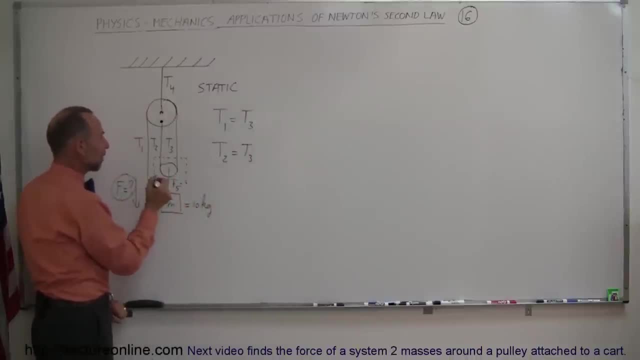 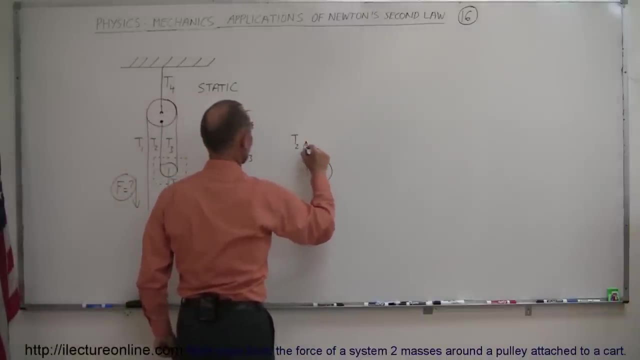 And finally, when we look at these three tensions, notice that if we draw a free body diagram, let me put it over here. So here's that bottom pulley, Here we have T2 in an upward direction, Here we have T3 in an upward direction. 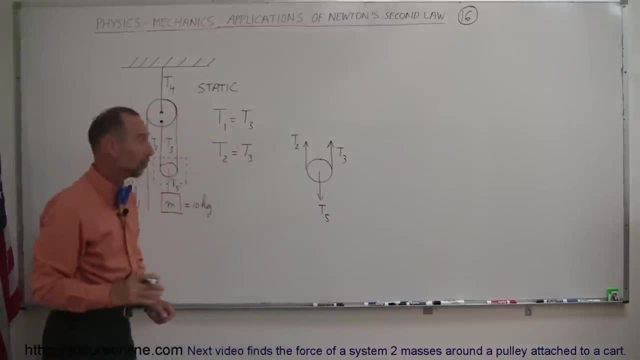 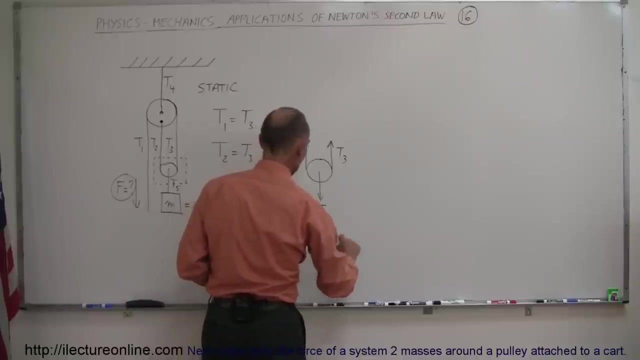 And here we have T5 in a downward direction. Notice that, since this is a static situation, all the forces in the upward direction must equal all the forces in the downward direction, so that there's no net force in the Y direction, which means that T2 plus T3. 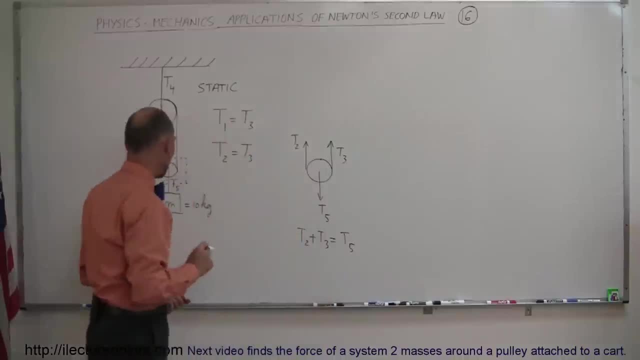 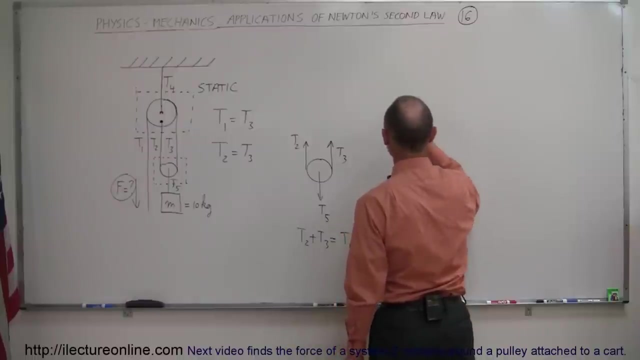 must equal to T5 in magnitude. All right, so that's established now. Now, if we look over here, here we can see that if we draw another free body diagram, put it right here we have one tension coming up this way: 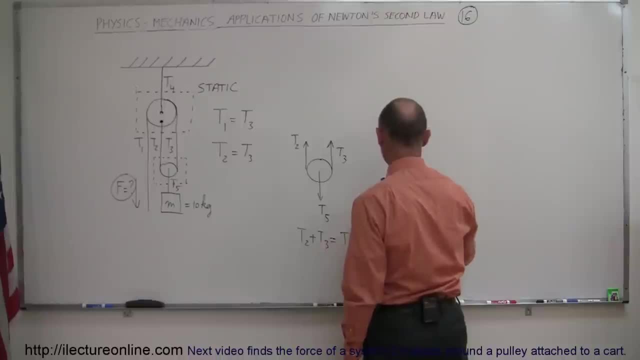 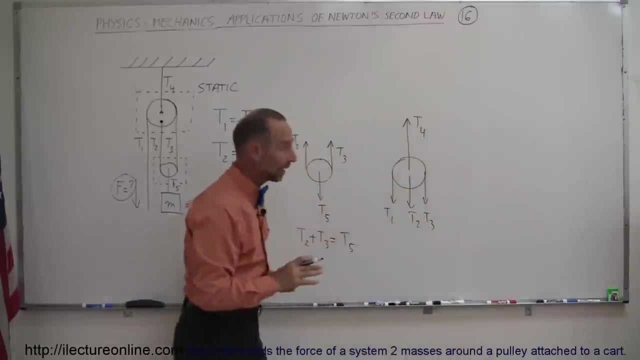 which is T4.. We have three tensions downward, so we have T1.. We have T2. And we have T3.. Again, since this is static and there's one force pulling this up, there's three forces pulling down. 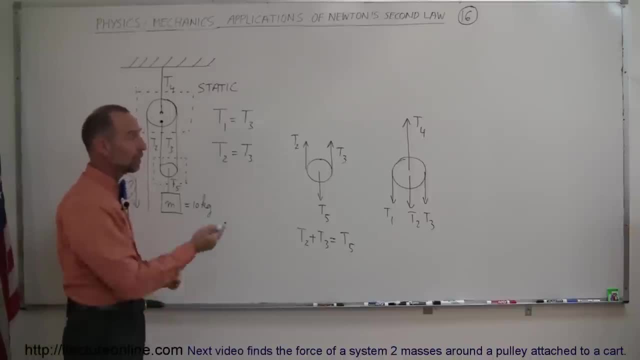 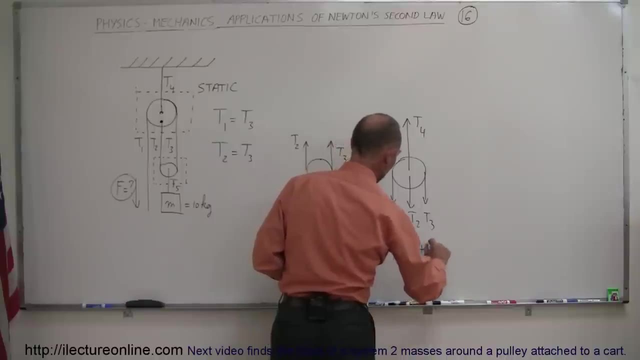 Again, you can say that since it's static, there should be no net force in the Y direction, which means that the force upward- T4, must equal the three forces downward- T1 plus T2 plus T3.. So now we have all the relationships. 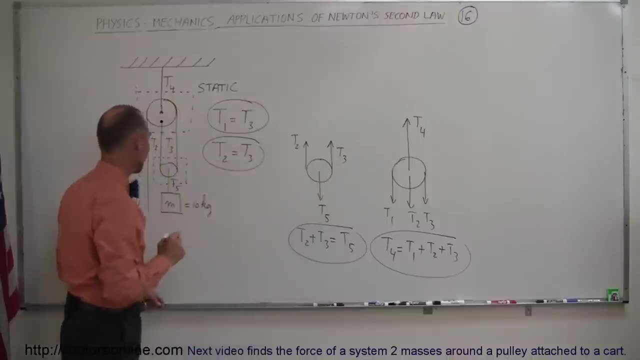 here and here. So now we can say: well, T5 must equal to the weight hanging from that pulley, which is the weight of that 10 kilogram mass, And I'm looking for my red pen right here. So this is equal to Mg. 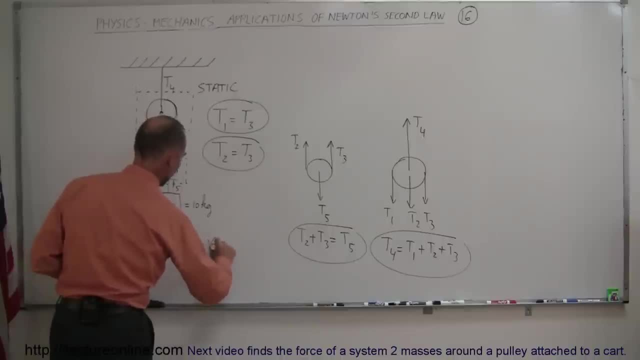 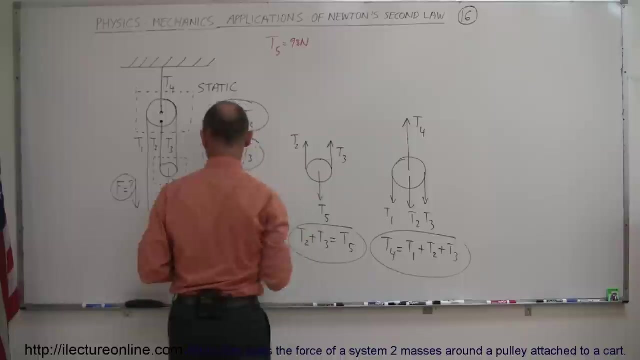 which is equal to 10 kilograms times 9.8 meters per second squared. So this is equal to 98 newtons, which means that T5 must equal 98 newtons. So that's one of them. So T5 is equal to 98 newtons. 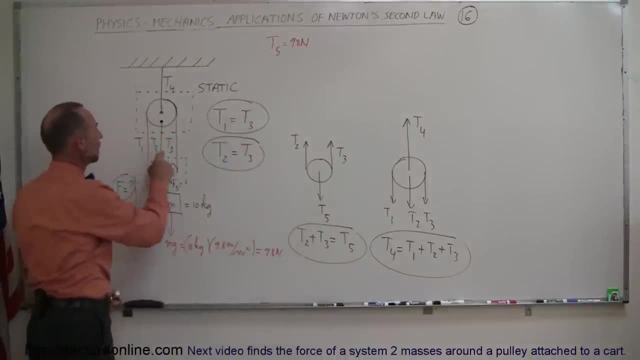 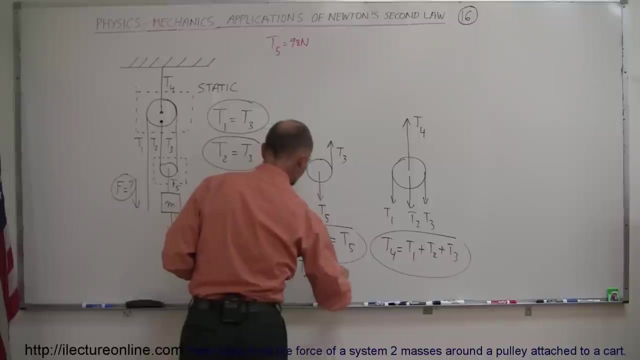 All right Now. we know that T2 and T3 must be equal and we know that the sum of those two must equal T3. T5 like that, which means that we can replace T2 by T3. So we can have T2 plus T2 is equal to T5,. 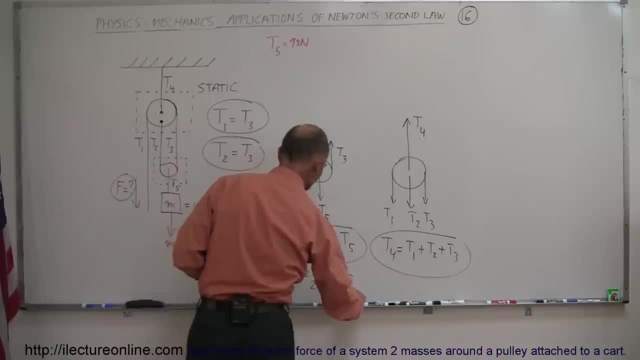 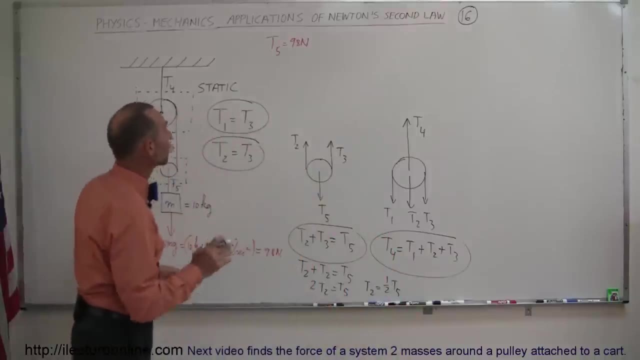 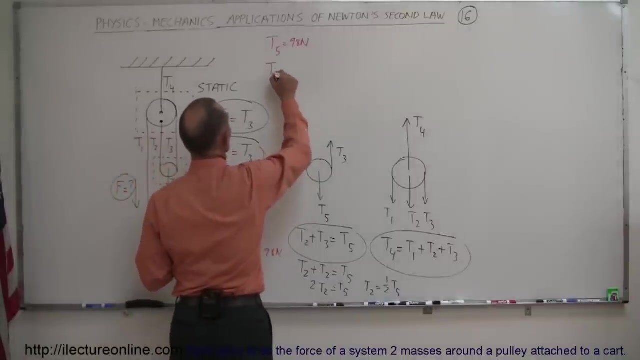 which means that 2T2 is equal to T5, or T2 is equal to one half of T5.. So since T5 is 98 newtons, T2 is half of that, which is 49 newtons, And so we can say that T2 is equal to 98 newtons. 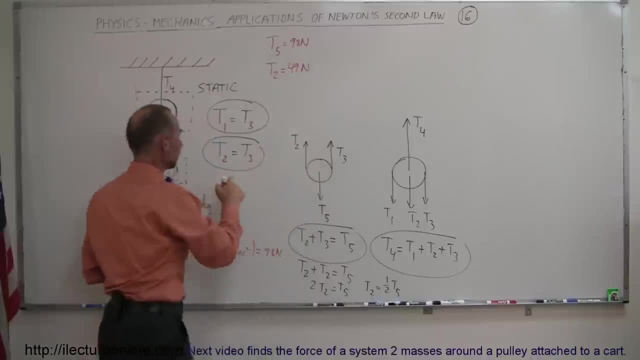 So we can say that T3 is equal to 49 newtons, half of T5.. And since T2 and T3 are equal, we can say that T3 must therefore also equal to 49 newtons. And then we see here that T1 is equal to T3. 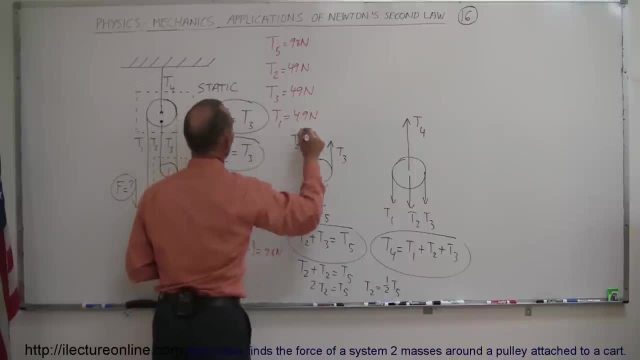 That means that T1 is equal to 49 newtons. And now we come up here and say that T4 is equal to the sum of T1,, T2, and T3, which means that it's equal to the sum of these three. 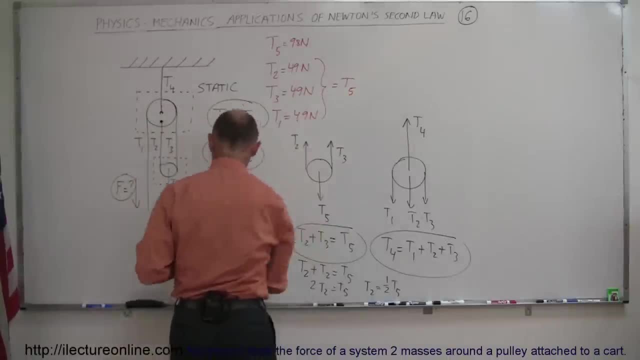 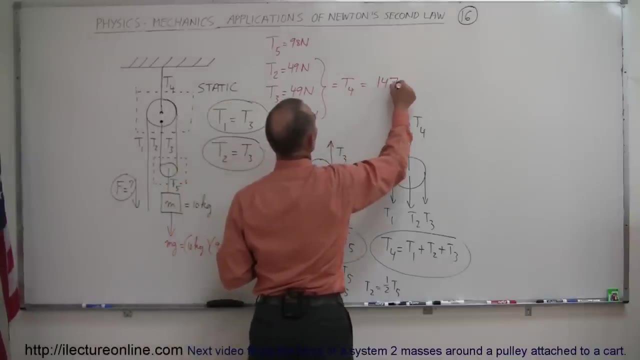 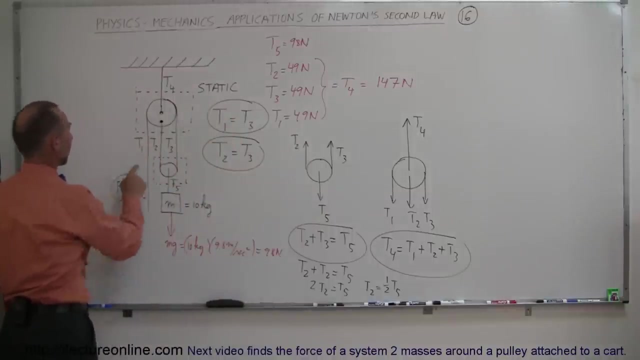 So this is equal to T5.. Oh, not T5, T4.. I got the wrong sum. I got the wrong subscript: T4. And so this is equal to 147 newtons simply adding those three together. Now how much force is required to keep everything in place?